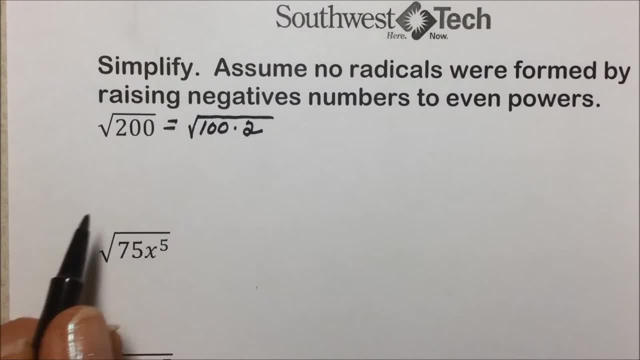 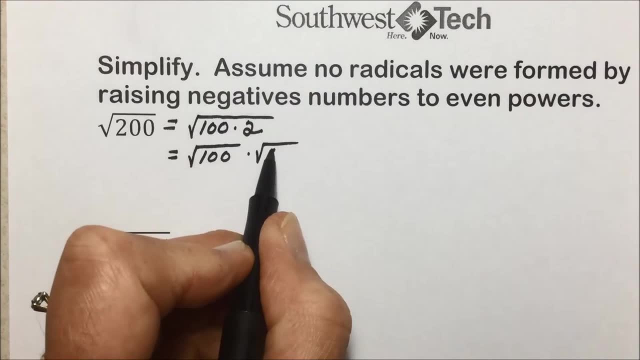 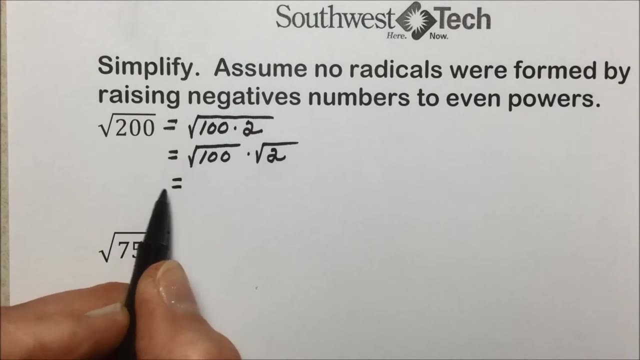 Then, using the product rule, we can break this into the square root of each of those factors and simplify it from there, The square root of 100,. since it is a perfect square, since 10 times 10 equals 100,, we can replace square root of 100 with 10 and leave the square. 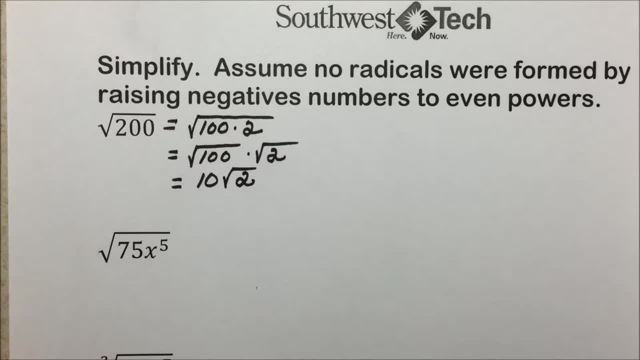 root of 2, as is, there is only one: 2.. This is known as simplified radical form. In the next example, using that same technique, looking for the largest perfect square here, since 75 is 25 times 3,, we can. 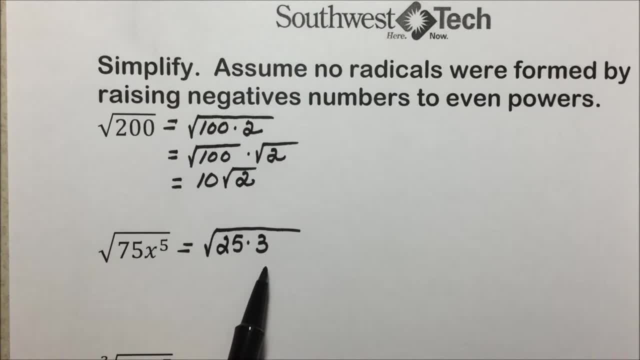 replace 75 with 25 times 3.. Looking for perfect squares here in terms of the variable x to the 5th can be broken down into an x to the 2nd times an x to the 2nd times an x, If you. 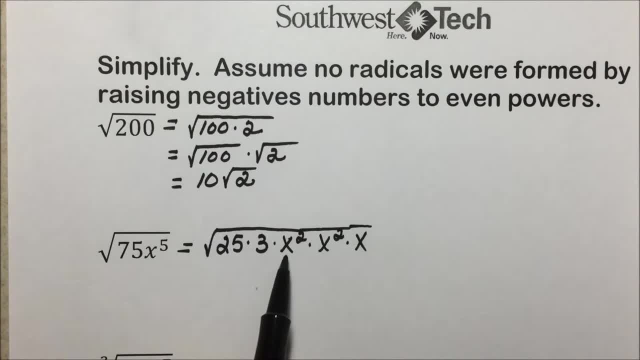 multiply those common bases together. we do have the equivalent of x to the 5th power. Now we can take the square root. I'll put the 25 and both of the x squares underneath one radical and the values or the factors that aren't perfect underneath another radical. We still have the same factors. This: 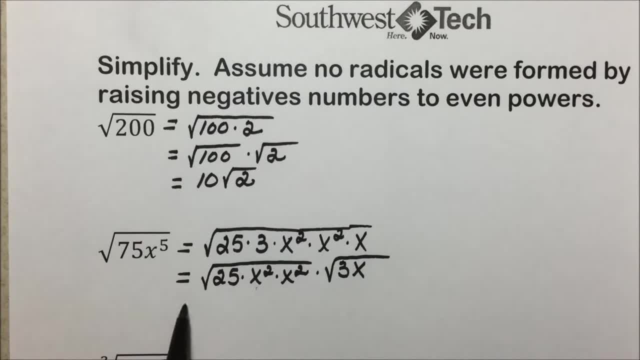 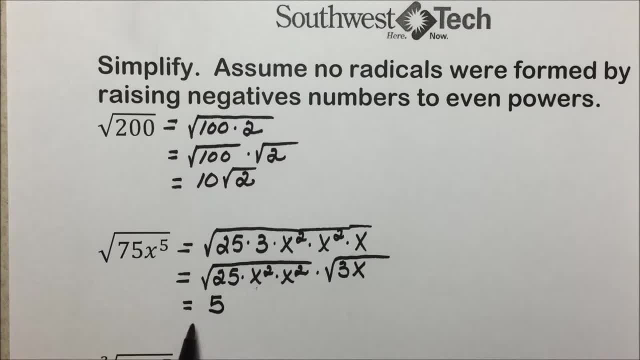 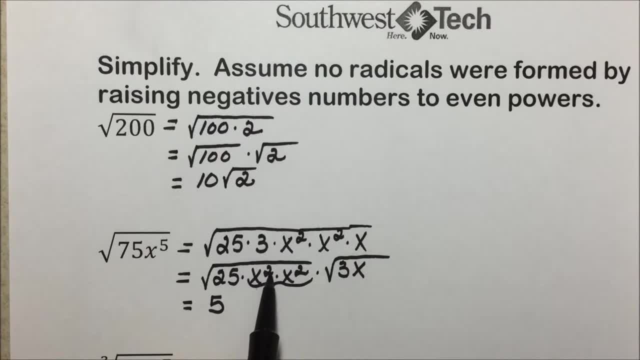 is 25.. We have two or a pair of x squared, so the square root of x to the 2nd to the 2nd is x to the 2nd and leaves us with the radical that we can simplify with the radical of 3x. 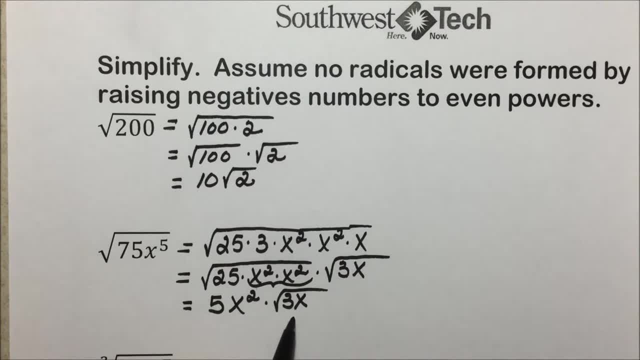 So our final answer here is 5 x 2.. x squared times the square root of 3x. Another way we could have gone with simplifying this is the square root of x squared- would have brought an x out in front. The square root of x squared. 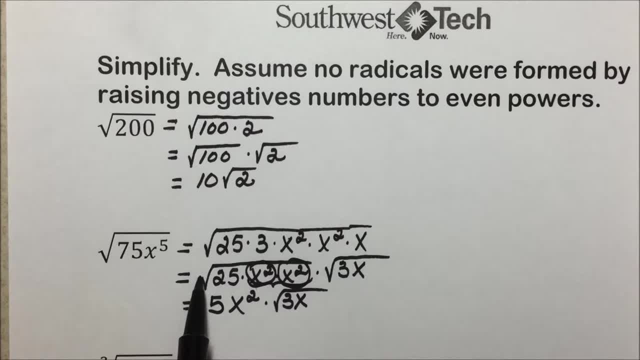 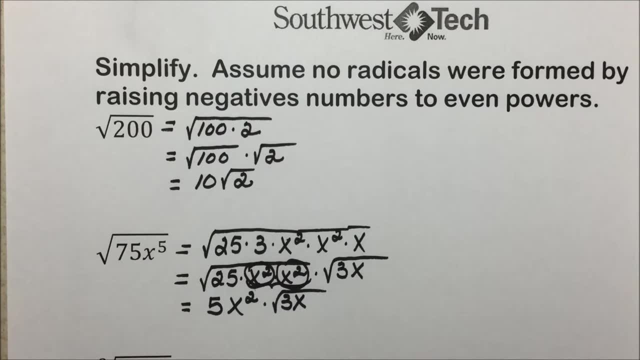 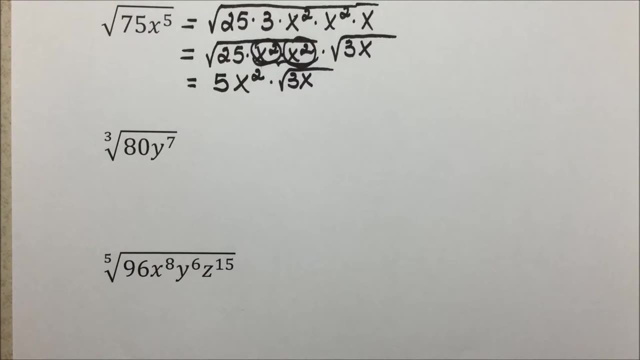 would have also brought an x out in front or out from underneath the radical. Those two x's, x times x, would result and simplify into an x squared. In this next example we have a cube root. Now we're looking for perfect cubes, The largest perfect cube, that is a factor of 80. 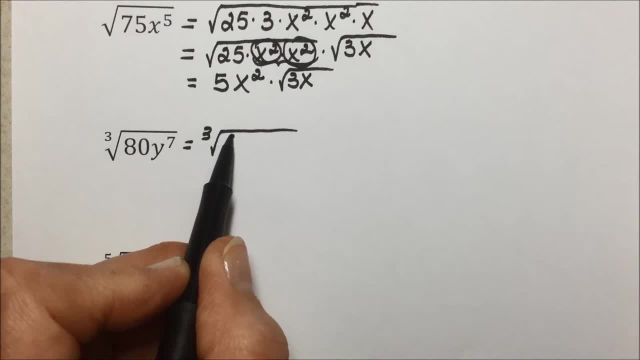 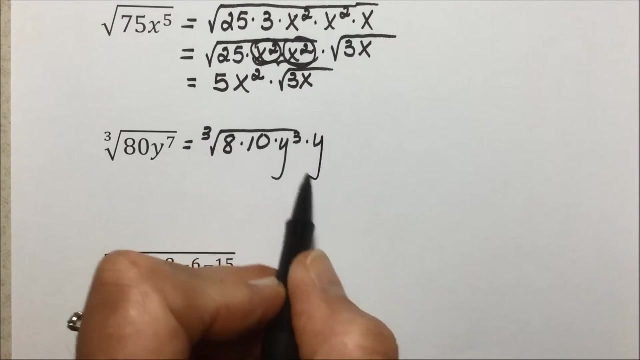 would be 8, and 8 times 10 is 80.. Looking for a perfect cube for y to the 7th. we could break that down into y to the 3rd, another y to the 3rd and a y. 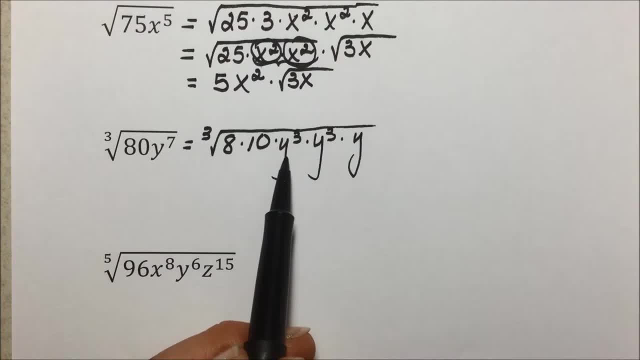 all underneath the radical. here Again, verify common bases multiplied together. Add your exponents: 3 plus 3 plus 1 brings us back to the 7th And just as a shortcut, then instead of separating out these factors into two radicals, we can just simplify from here. The cube root of 8 will give us 2.. Cube root of 10,. 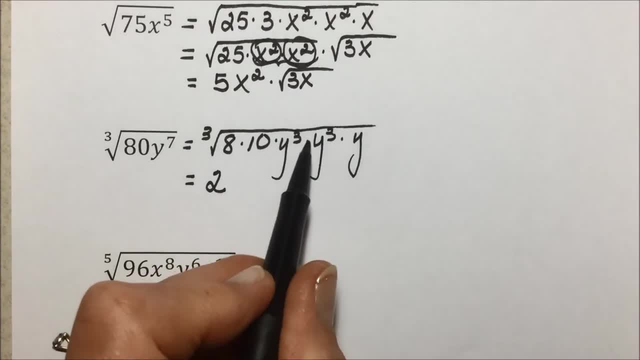 we can't do anything with. It will remain underneath the radical Cube root of y to the 3rd. We have another y to the 3rd power We'll bring out a y Cube root of y to the 3rd brings. 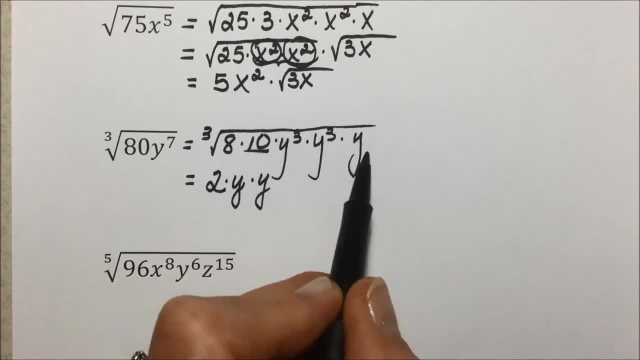 out another y And we're still left with y to the 1st power. So 2 is the square root of 8, y to the 3rd. the cube root is y same with this other one And left underneath the. 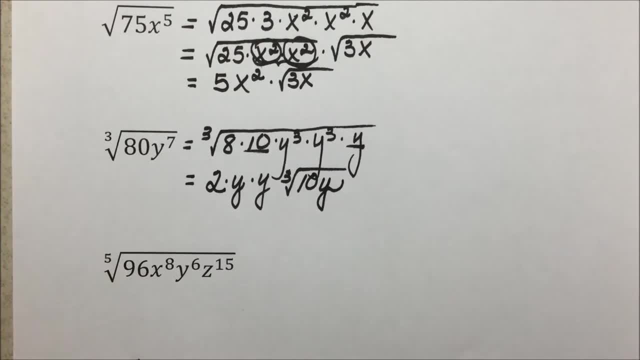 radical is the 10 and the y. If you're having difficulties seeing where y to the 3rd is is coming from, we could take this a step further and let me show you the entire prime factorization of this radical cube root. we're looking for three of a kind. 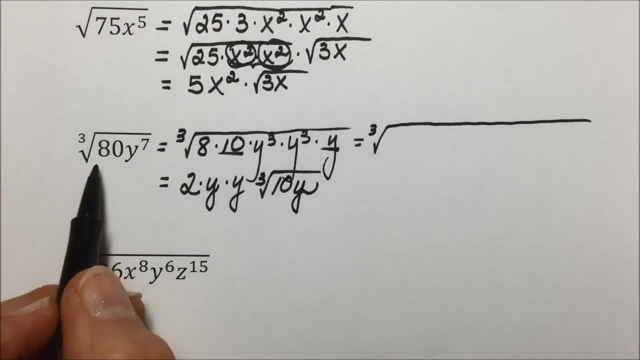 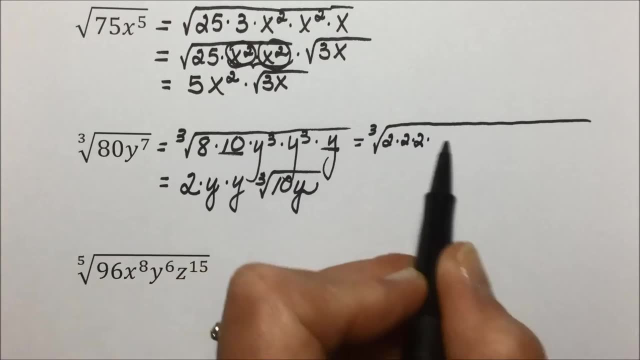 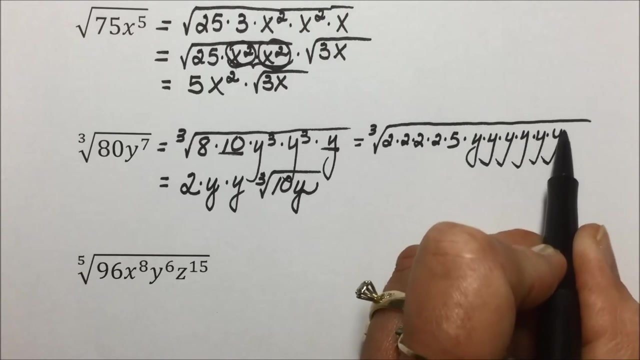 and let me get my radical long enough here. if we do a prime factorization, eight would break down into two times two times two. ten is two times five, and then we have seven eights multiplied together, or seven y's multiplied together. so let me get seven Y's, multiply it here and I think I have them. two, four, six, seven. 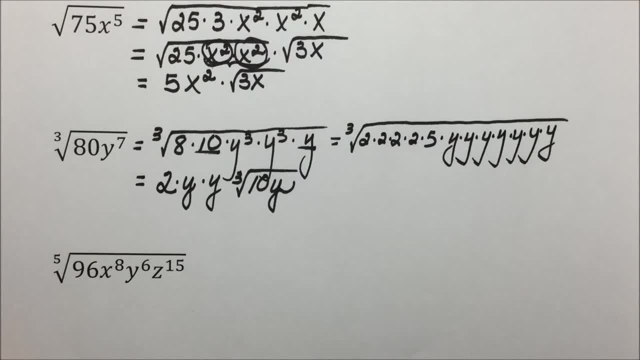 all right now, when we're looking for a cube, we're looking for three of a kind. so here is a three of a kind. what times itself? three times is equal to what originally was. the is equal to what originally was. the root of these three factors brings out a 2.. We only have one 2,. we only have one 5.. Again. 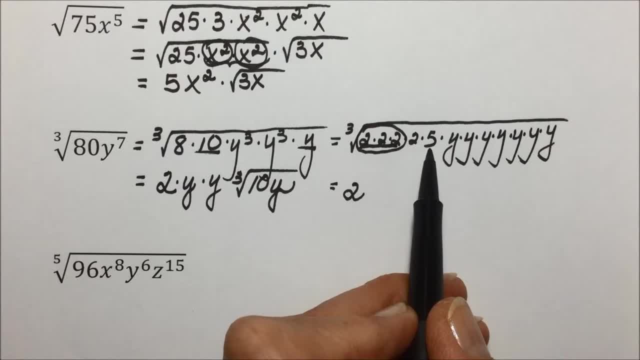 we're looking for 3 of a kind. Here is 3 of a kind, which means out comes the y. Y is the cube root of y. to the third power. Here's a group of 3. That will bring out a y as well. 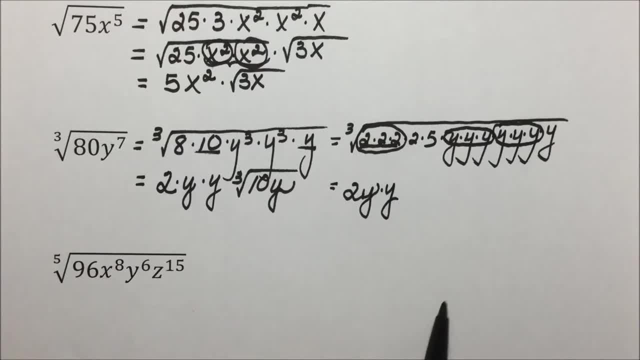 And we still have only one y remaining. So here's that value left underneath the radicand, the 2 times 5 times y or the 10y, And cleaned up, we most likely would write 2y to the second. 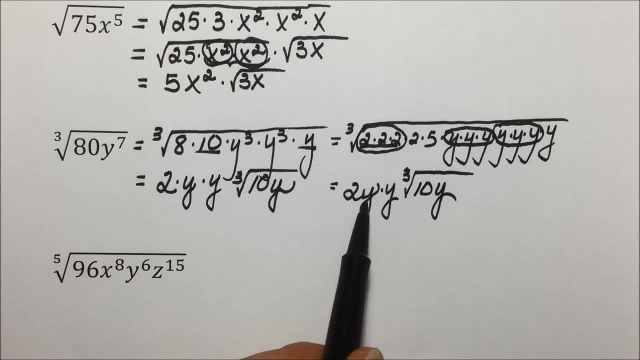 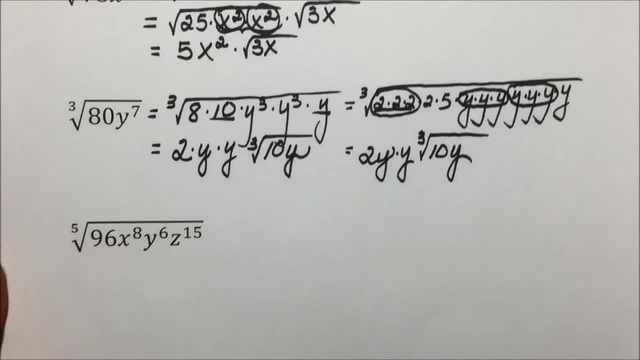 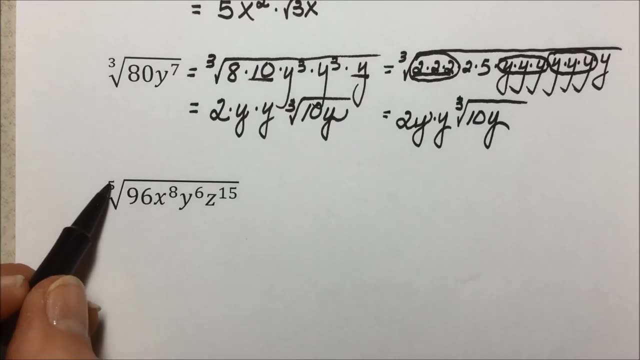 power times, the cube root of 10y. for our final answer. In this next problem we're going to look at how to solve this problem. In this problem we are looking for the largest perfect fifth root that goes into 96.. And 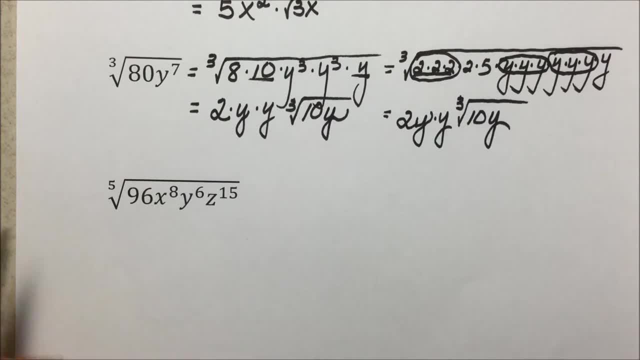 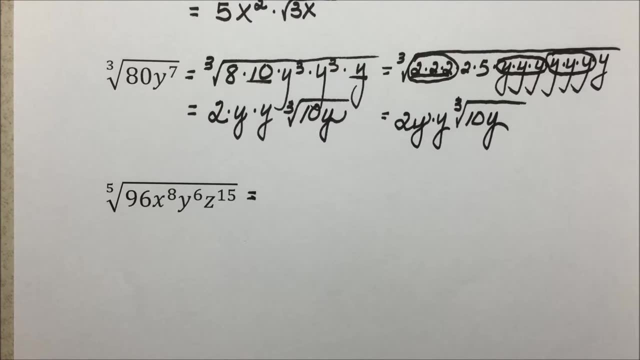 if you do some calculating it turns out that there are a bunch of 2s in 96. And to help with that you can do your prime factorization And it turns out that that ninety-six is the product of thirty-two times three Thirty-two. if you break that, 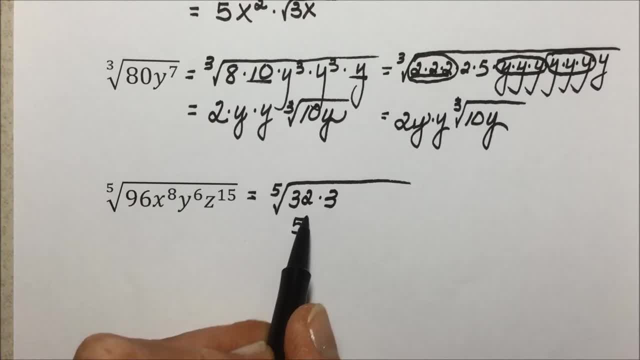 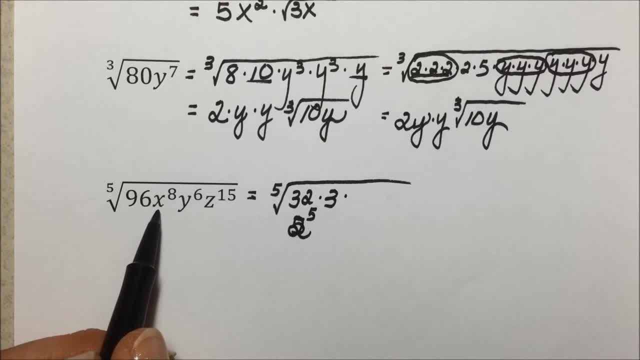 came from. but let me try it again: x to the eighth power is x to the fifth times x to the third. if I break it into a perfect fifth root, y to the sixth. I'm going to break it into a y to the fifth, with a y to the first. 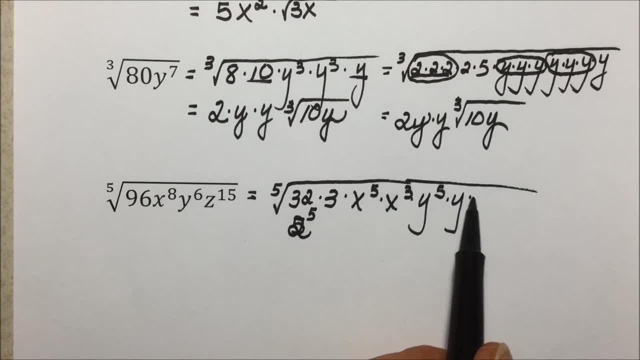 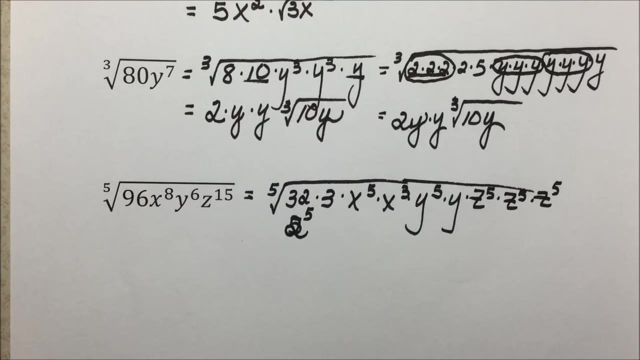 1st and a z to the 15th. we can have 3z to the 5th which multiply together to give us our z to the 15th. So we have it broken down to help you see it visually. The 5th root: 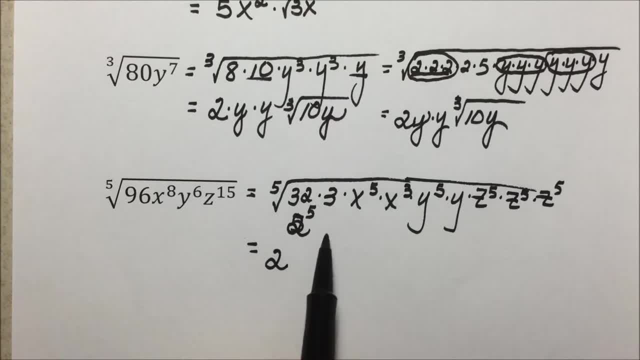 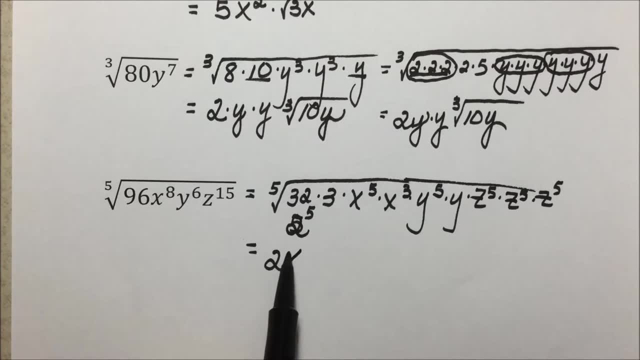 of 32 is a 2.. There's only one, 3, we'll leave that underneath the radical. The 5th root of x to the 5th means x is the perfect 5th root, x to the 3rd, not high enough power. 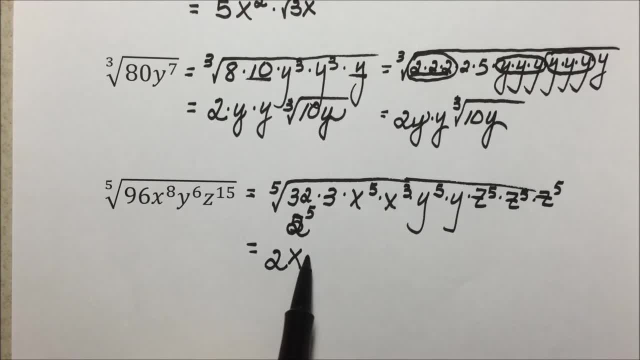 but y to the 5th is The 5th. root of y to the 5th is a y. not enough with the y, and each one of these z to the 5ths will bring out a z for each one of those leaving those. 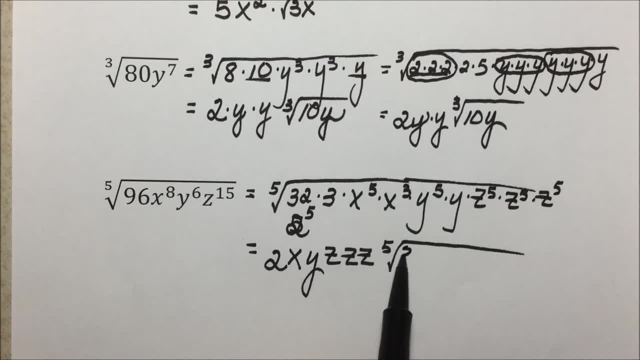 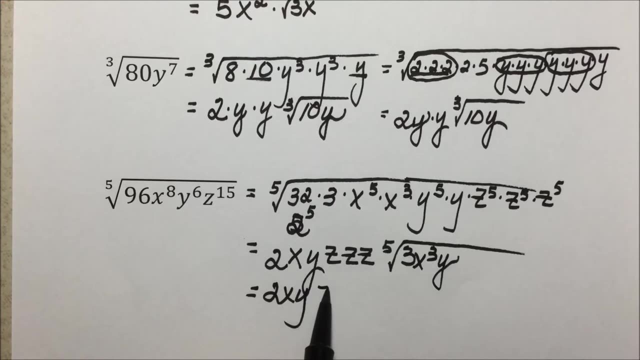 factors that didn't have high enough powers. We have the 3,, we have the x to the 3rd power and the y. We can simplify this: instead of writing 3z's multiplied together, we can write this as 2xy. z to the 3rd power, 5th root. 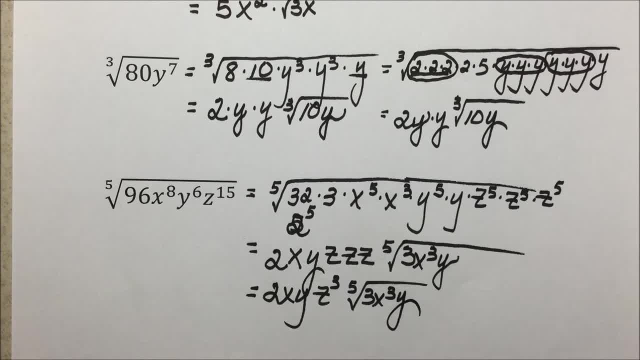 of 3x to the 3rd power, y, underneath the radical. Now we can convert these radical forms into rational exponents. and try to do this mentally. If you're noticing what's happening here and using the conversion to a rational exponent, I'm going to ignore the 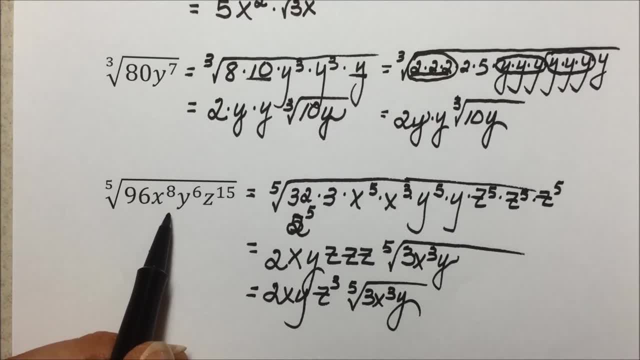 number right now, but looking at just the variables as a shortcut here, this is 96. x to the 8th, y to the 6th, z to the 15th. is this whole quantity is to the 1st root of? 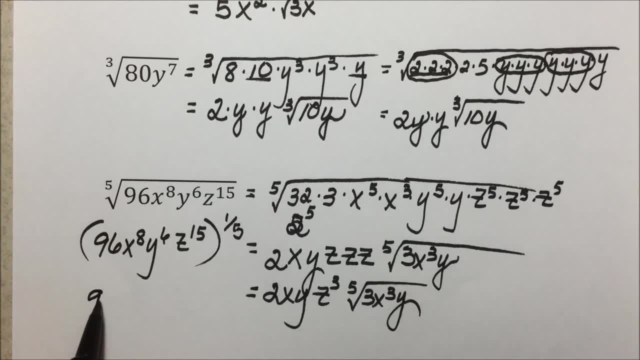 the 1st power- And, as I said, I'm going to ignore the 96- to the 1, 5th power. We handle that here by using our prime factorization. But if you look at the exponents and what we have is a product raised to a power, So each one of these is raised to that 1, 5th. 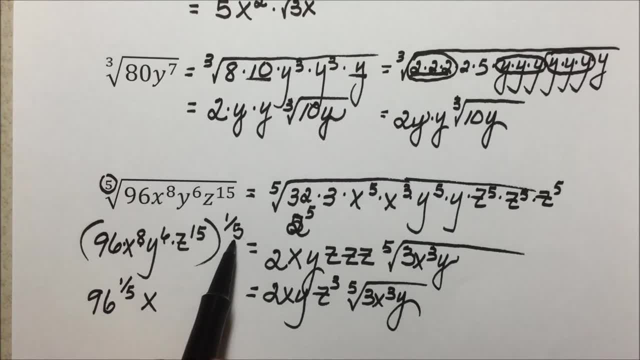 power, The index becomes the denominator of our rational exponent. So we have x to the 5th power and we have a product raised to a power. So each one of these is raised to the 1, 5th power. So we have x to the 8th raised to the 1: 5th, a power raised to a power. we. 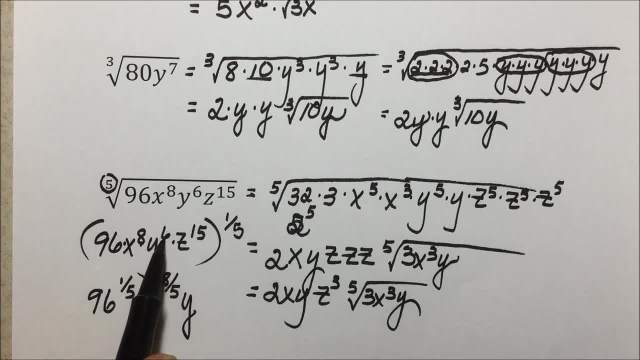 multiply, which is 8 5ths. Likewise, y to the 6th, raised to the 1, 5th, you multiply 6 times: 1: 5th is 6 5ths and z to the 15th times, 1 5th, 15 5ths gives us a 3.. If we go, 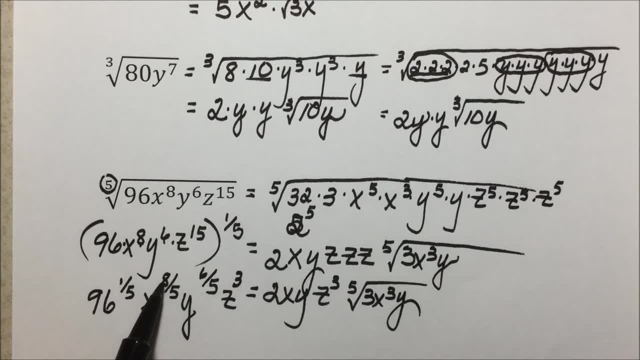 back and we simplify this: how many times does 5 go into 8?? 5 goes in once, with 3 left over, And here's what we ended up with. Here's our x to the first. We have a whole group of 5 x's multiplied together, which is the 5th root, and 3 were 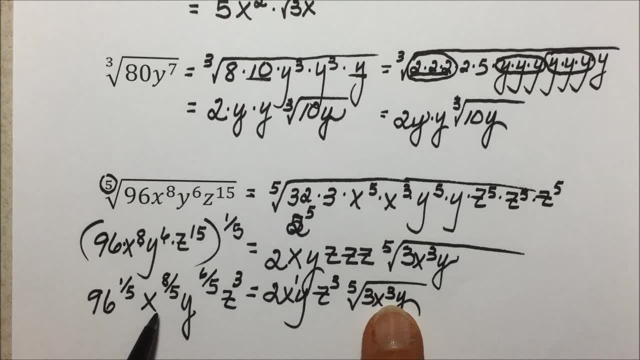 remaining And notice what's underneath: the radical x to the 3rd power. When we move to the next one, y is to the 6th 5th power. when we're taking the cube root of this, radicand 6 divided by 5 is 1.. In other words, there's 1 x to the 5th power, So we have x to the. 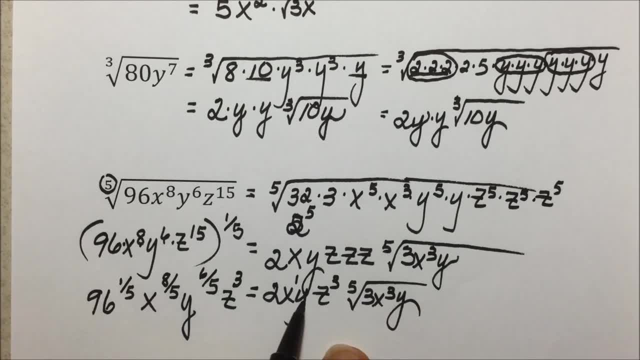 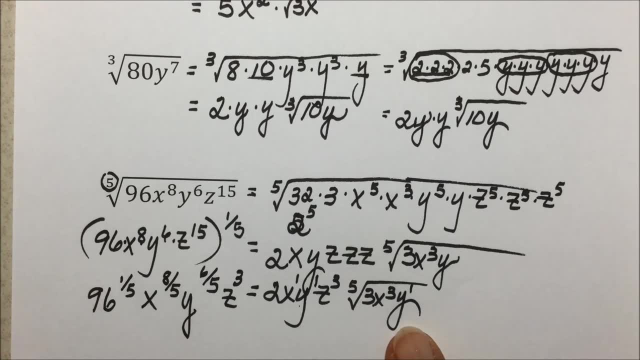 1 group of 5 y's multiplied together and here it is y to the 1st power with 1 left over, and that 1 left over remains underneath the radicand radical sign. in the radicand And the last one we had z to the 15th times. 1, 5th, 15 divided by 5 is z to the 3rd and